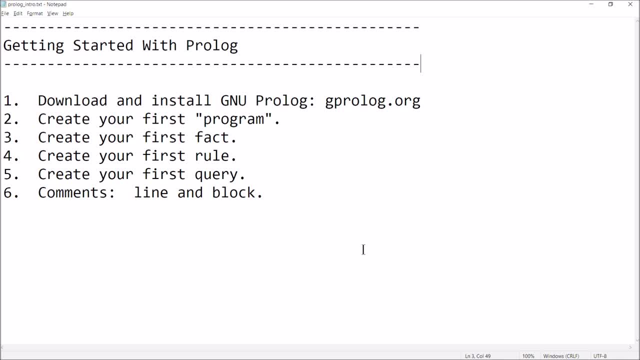 And then, as part of that first, like I said- quote program, I'm going to show you how to create a fact, show you how to create a rule and show you how to do your first query, which is just asking your Prolog interpreter, asking your knowledge base, to answer some kind of question for you. 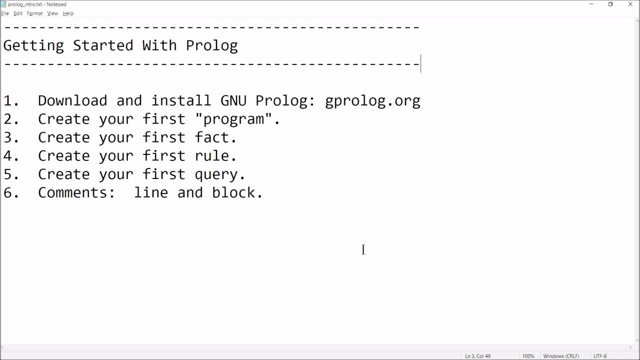 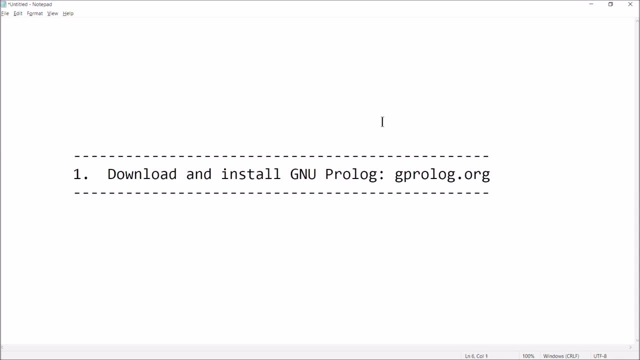 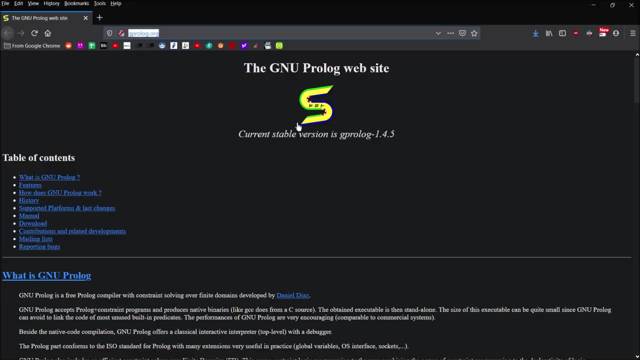 And then I'll just finish off briefly show you how to do comments in Prolog. Okay, so let's go ahead and get started And let's go ahead and download and install Prolog, right? So we're going to go to gprologorg, right? 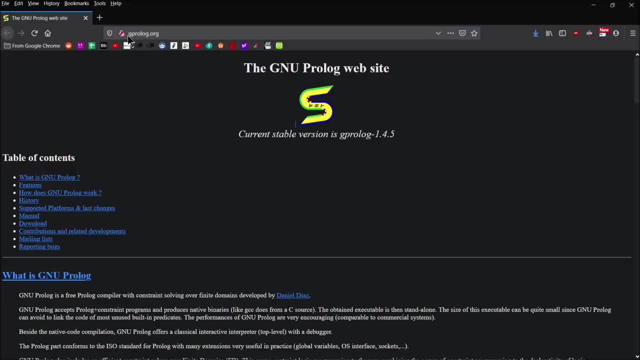 And so you can see that I already got this sucker loaded up. gprologorg, And this is what the website looks like. It's totally free. Download this, no problem. Click at table of contents. click on download. You're going to be given a bunch of options here. 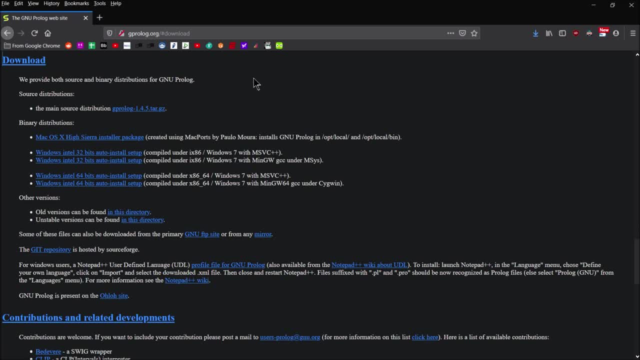 So you just want to pick the operating system that you're going to be working with, And for me I'm going to be. I'm going to be working on a Windows 64-bit system, So I'm going to click this link right here. 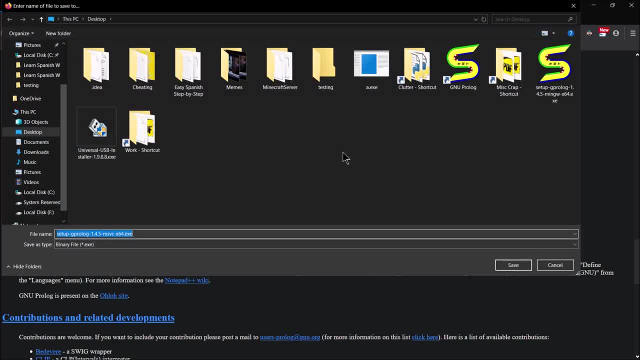 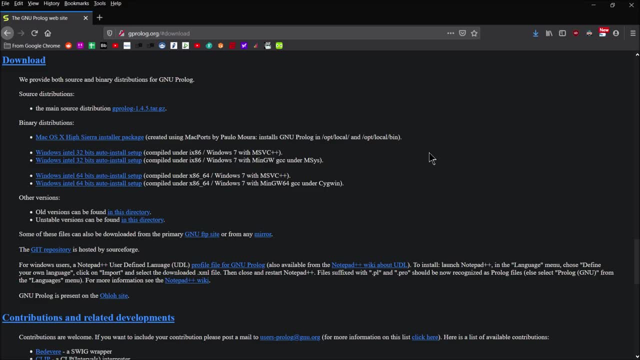 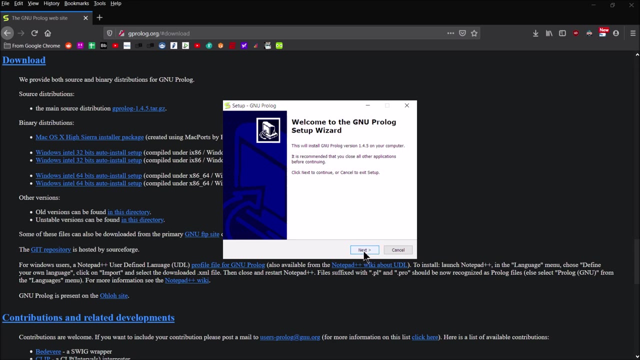 And I'm going to go ahead and save that onto my desktop And once that's done I'll go ahead and run that program right, And so you can go ahead and just install it, you know, to the default location and you know. 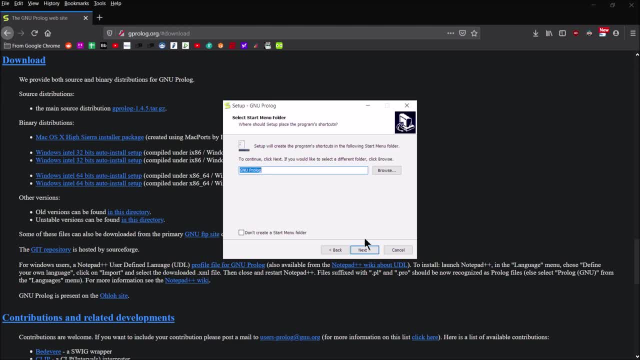 or wherever else you want to, Wherever else you want to put it, And you know that should be fine. I'm just going to create a desktop icon and then just do all the defaults here And you'll see that that install goes pretty, pretty quick, right. 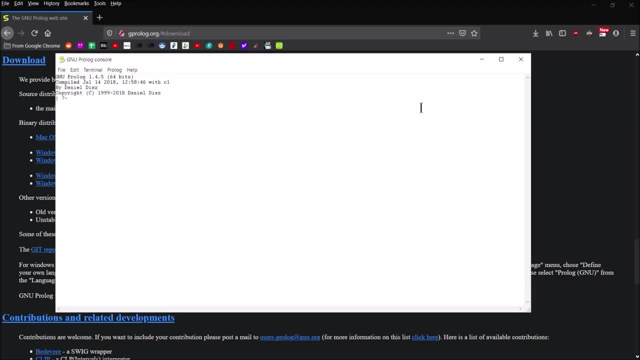 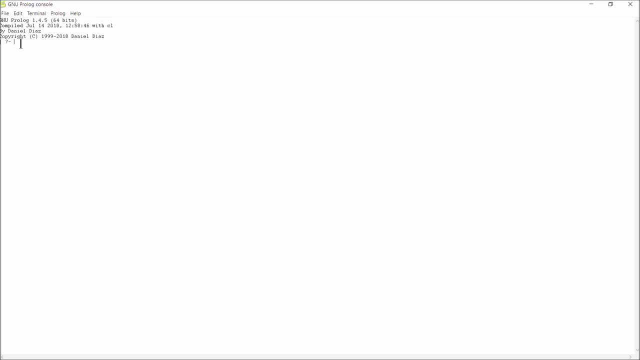 So when you're done, you can go ahead and click finish and launch Prolog And you'll see that we've got ourselves a console right. So in here is where we'll be able to type our Prolog commands. you know, load our knowledge basis. 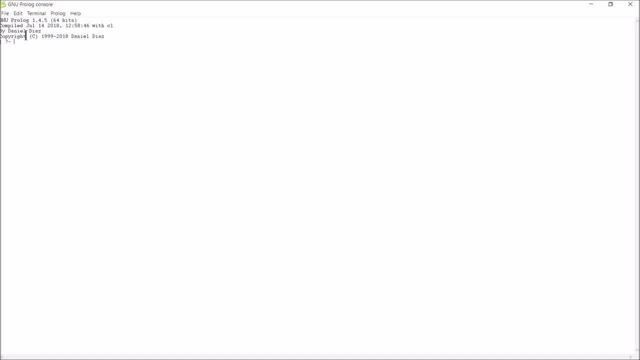 you know, do debugging et cetera right. So one thing you can do here if you want to make it a little bit easier to read is you can go under terminal change font. You know, I'm going to want this to be a little bit bigger. 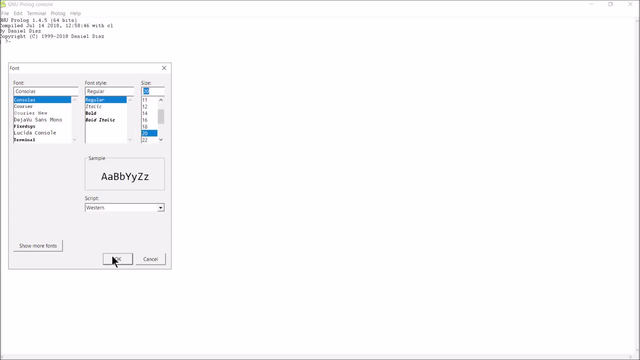 I like console-less font as opposed to Courier. I'll make it like 20 or something like that. You can see that the font gets bigger And when it comes time to load and run some code, you know we're going to need to go to file. 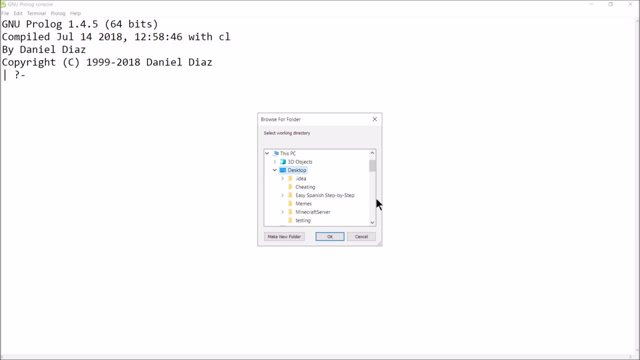 change directory and then point that to the file. that's got our code on it right. So we'll go ahead and hit okay And you'll see that it says yes, That means everything happened just fine. And change directory is a command, and this is where I wanted to change my directory to. 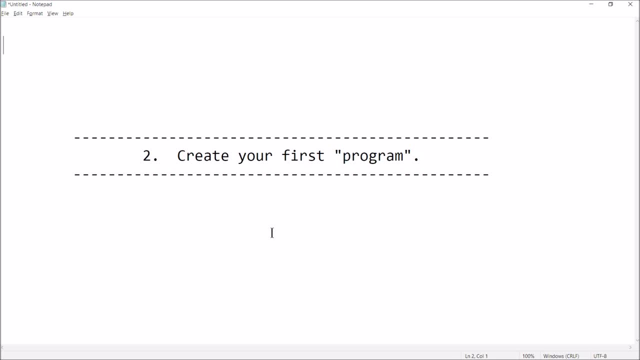 Okay, So let's go ahead and get started with our first Prolog program. okay, Now there's a couple different modes in which you can work within Prolog right, So you can go through the console right And you can use the Prolog interpreter. 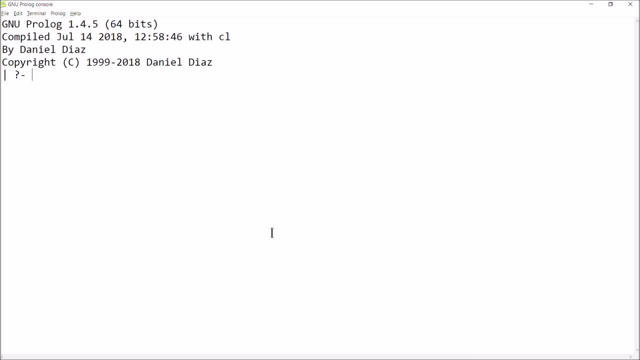 Prolog interpreter, if you will okay, So I could come here and you'll see that we got this question mark and this dash, This is the prompt, right? So the console here is trying to, or is waiting for us to, actually type in some kind of command. 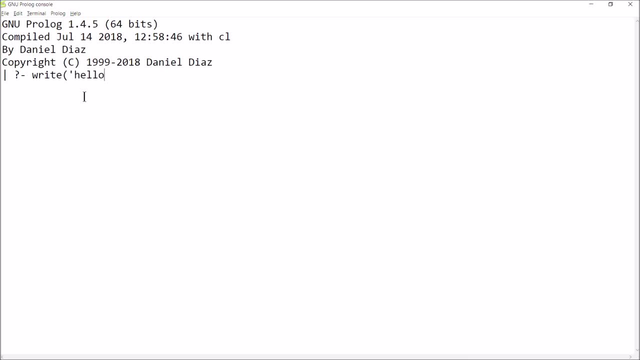 So, for example, if I wanted to put hello world on the screen, right, I could say: write hello world, okay, And that is a command, right, the write hello world. And to mark the end of that command I use a period right. 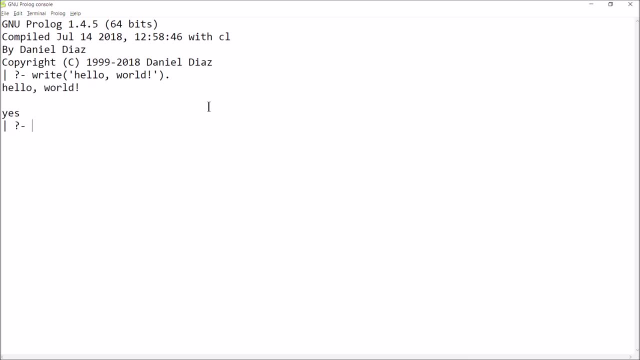 So a period is like the semicolon in the Prolog world. So if I hit enter, you know you can see hello world. You'll also see this yes here. So yes or true, those are both equivalent. Basically, what that means is: yeah, everything went great. 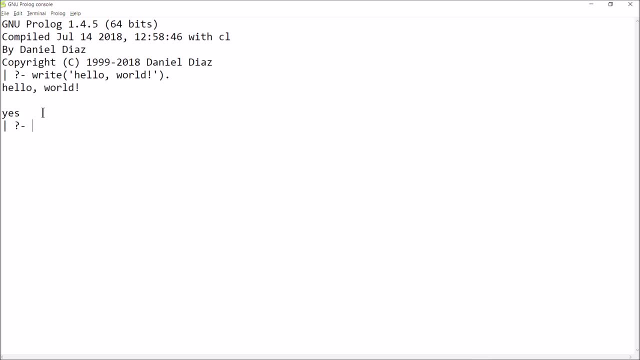 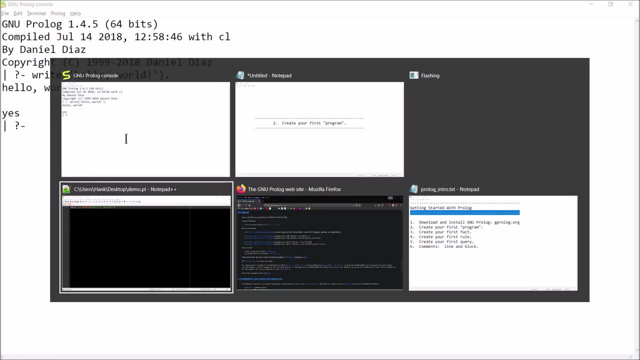 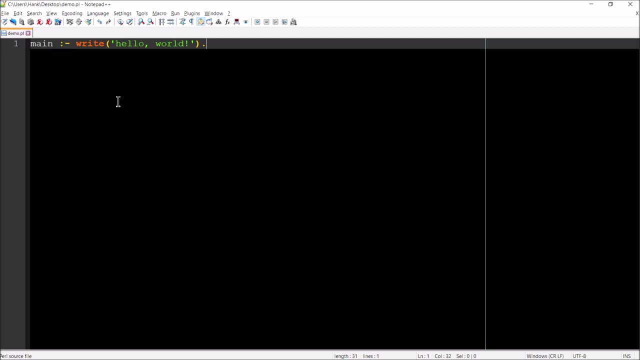 I ran the query. It was successful. Everything is awesome, Okay. So another way you can run this is to: Okay, You write your own source code file And, as you can see up here in notepad, I named this thing demopl. 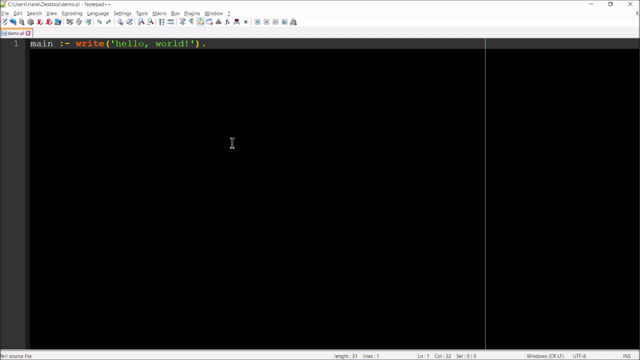 And this first line right here is an example of a rule. More on this in just a bit. But essentially what I'm saying is: look, I want to write hello world And you know, I'm going to run a query that you're going to match. 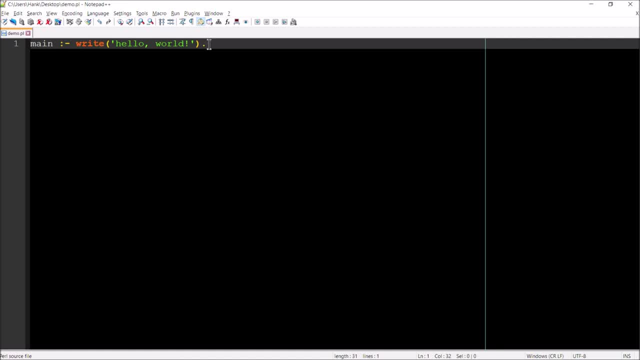 And when you match that query, you're going to execute this command, right, Okay? So let me show you how that works. So what we'll have to do Is we'll have to load our knowledge base. That's what's in here. 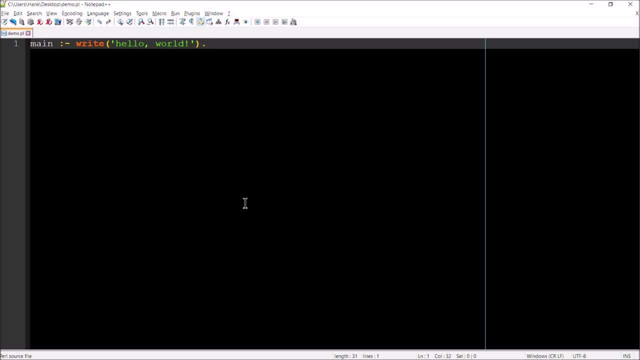 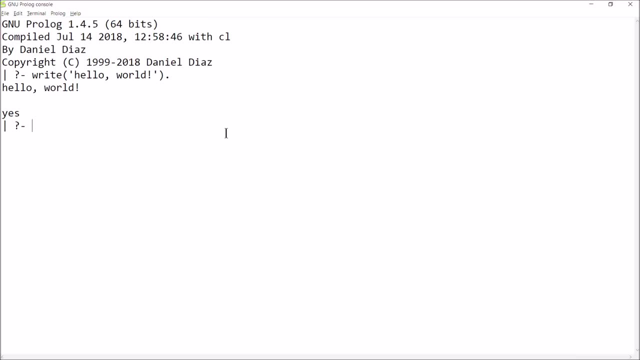 Just this one line, Just this one rule Into the Prolog interpreter And then we'll be able to run a query which will cause hello world to happen on the screen, And I'm going to show you how to load that file. So that file was demopl. 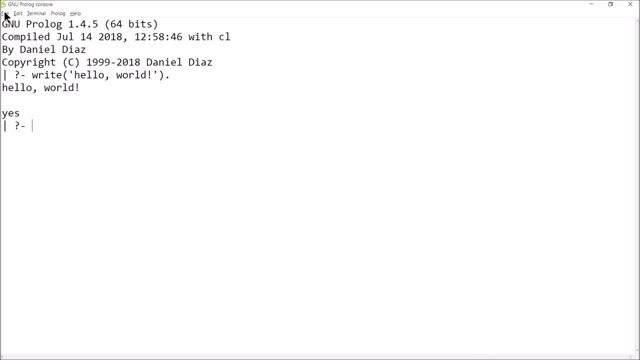 Okay, And I have that saved on my desktop And so I'm going to use file change directory to get into the same location as that file. I'm going to hit okay, Okay, And you'll see the response here: Change directory. 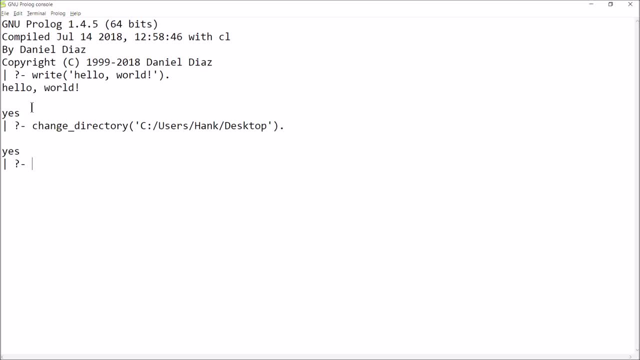 I could have typed all that out, But the console allowed me to do this kind of automatically, And so now I can load that file into the interpreter, Right. So the name of the file is demopl. I can just type in demo inside these square brackets. 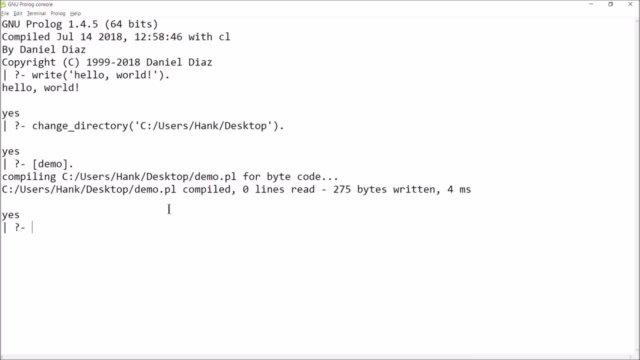 You know, hit my period, Hit enter And you can see: look, I'm going to go ahead and compile this thing, And then we're ready to go. Okay, So now, if I want to see that hello world, I can run a query. 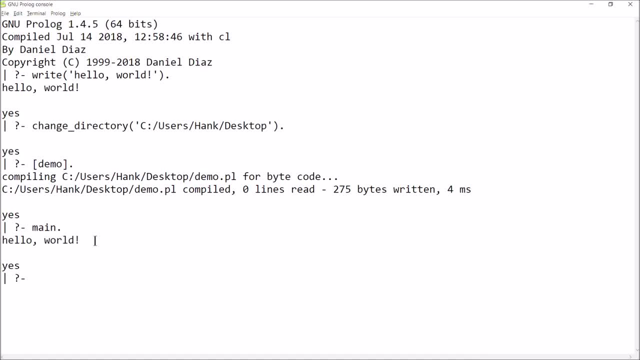 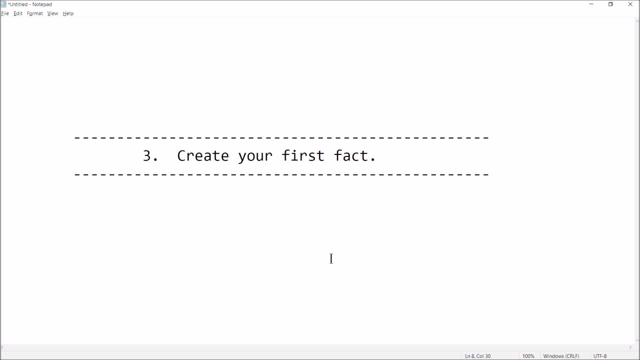 Just type main period, Hit enter And you can see there's the hello world. Okay, So next up, let me show you how to create a basic fact. So prologue your source code. you're making a knowledge base. 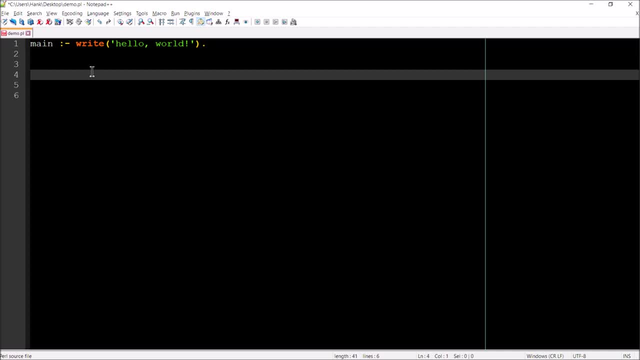 Knowledge bases are facts and rules. So if I wanted to create a fact that was relating a couple of things to each other- for example, you know, maybe I wanted to state that you know, California is next to Nevada- Okay, So this would be an entry that I would have inside my source code and a statement, as it were. 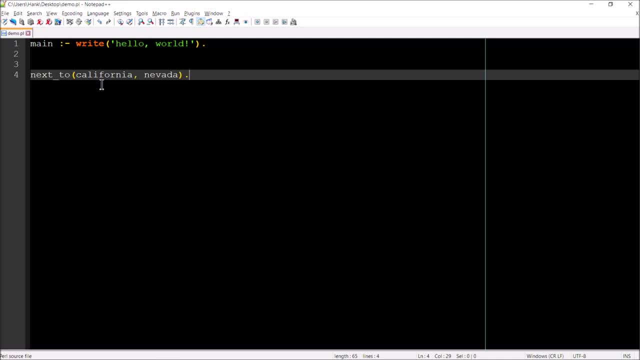 And I'm creating something very similar to what you see in predicate logic, where I'm setting up a relationship So next to- and the arguments inside the parentheses are relating saying California And Nevada are next to each other, Right? So it's a fact. that's got a couple of elements inside this function, like syntax. 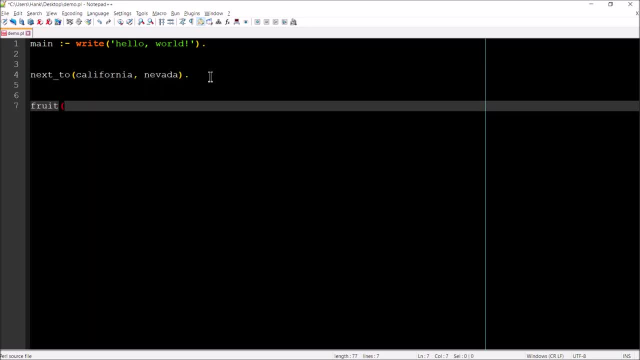 But I could also say: fruit, orange Right. So if I do that, I've just got the one thing inside the parentheses And I'm saying, hey, a fruit's an orange Right. Or I could say, you know, an apple is a fruit. 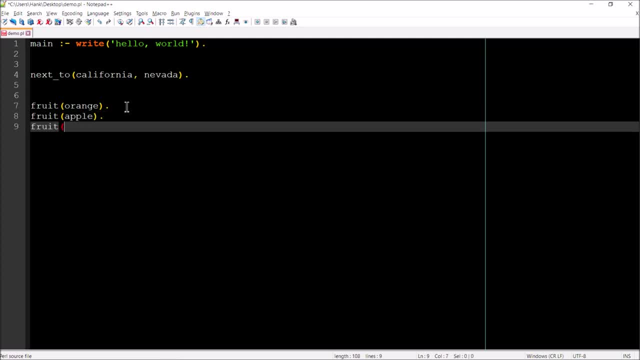 Or I could say that A pear is a fruit. Fine, You know. and then I'll add a couple more facts up here too, just to set up some quarters here. in a second. I could say: well, California is also next to Oregon. 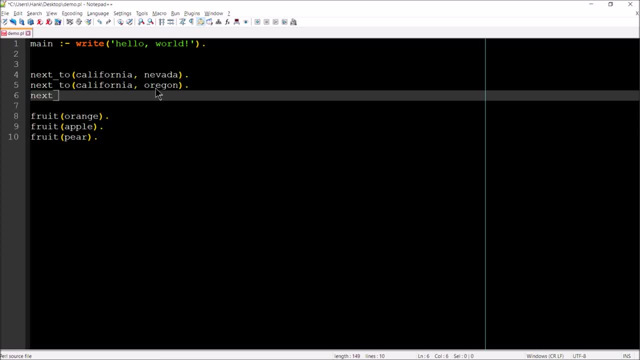 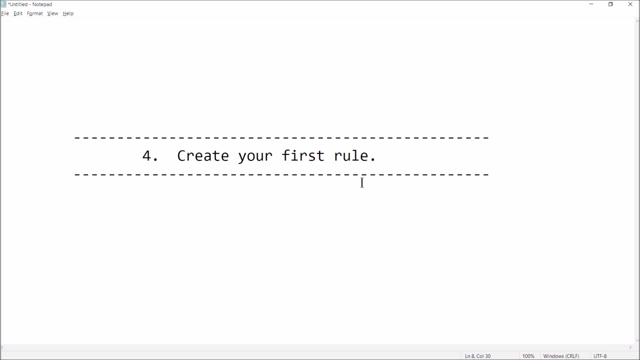 And I could say that California is also next to, you know, Arizona. Okay, All right. So next up, I'm going to show you how to create A rule, Maybe something a little bit more useful than what we had initially. 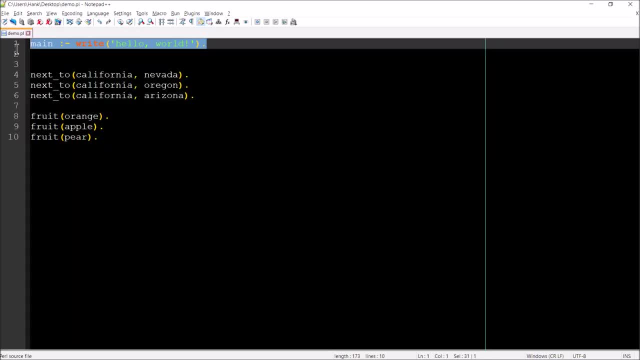 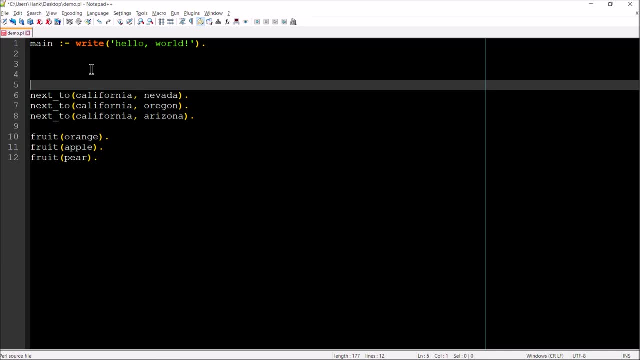 Right. So this guy up here on line one was a rule, Right. But what I'm going to do here is I'm going to add some additional rules and kind of explain in a little bit more detail what's going on. So if I wanted to see if it would be possible for me to travel from, say, California to Arizona, then I can set up a rule. 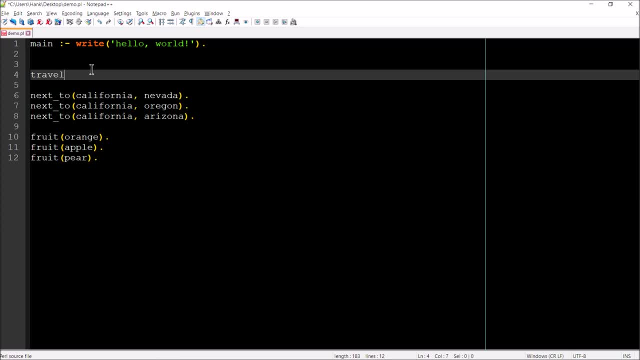 Right, And I can name that rule travel, Okay. And if I want to know if I can get from point A to point C, Okay, I'm going to type in. you know, I'm going to give a name for my rule here. 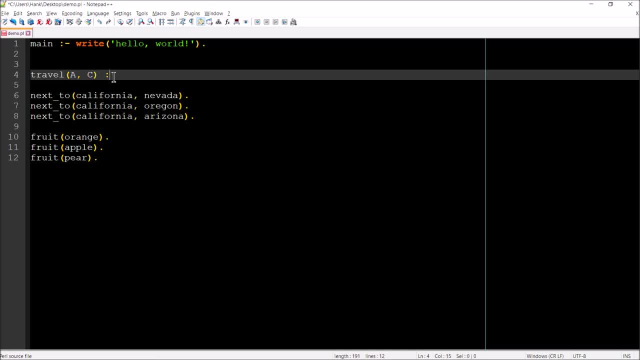 And I'm also going to say, well, I want to go from point A to point C. Okay, Now I also have this operator right here, the colon and the dash. Okay, And following that, what I'm going to have is I'm going to have: 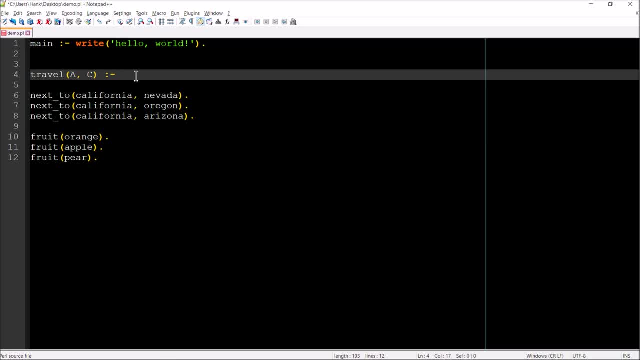 Okay, I'm going to have a couple of facts that are going to be built into this syntax, Right, So I can say: well, next to, and if we start off at point A and we go to point B, well then can I also get from point B to point C? 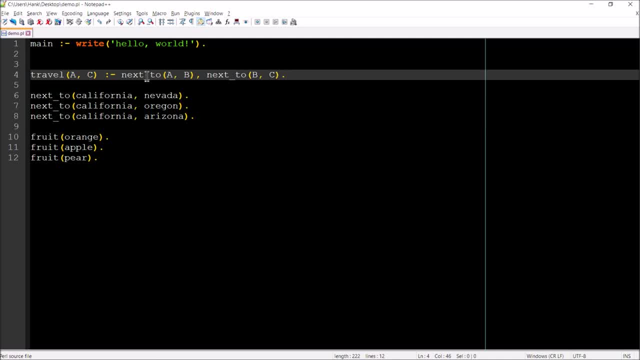 Right, So period. So this is going to allow me to see if I can travel, Say, from California to Nevada and then from Nevada to somewhere else. Okay, Now, in order for this rule in line four to work, then I probably should add a couple more facts here. 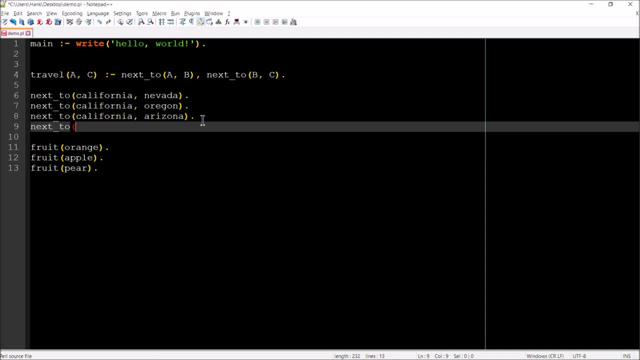 So I could say something like: well, I can go from Oregon to California. Right, I can go from, Oops, I can go from, Let's see here, I can go from Nevada to California. Okay, Oops, Nevada. I should probably just type here: 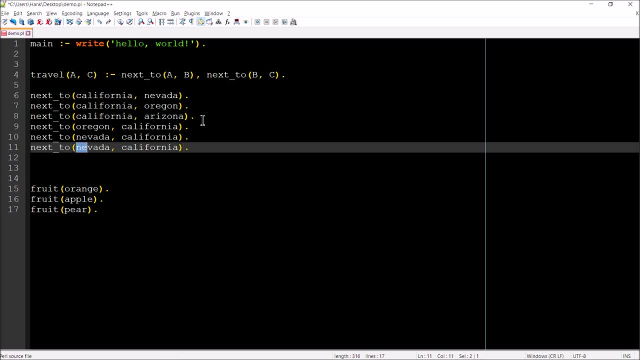 And I can go from Arizona to California. Okay, So line four is what a rule looks like. Added a few more facts here on lines nine through 11. And when we take a look at queries We'll see how this rule plays out. 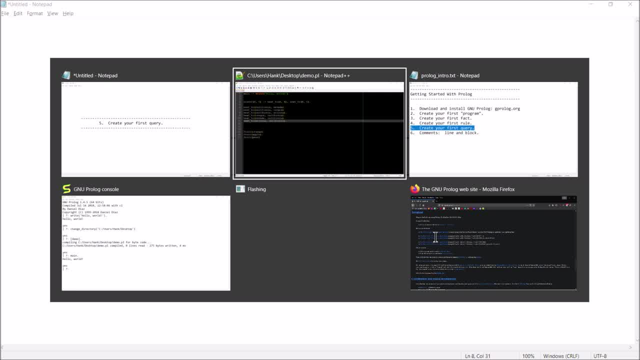 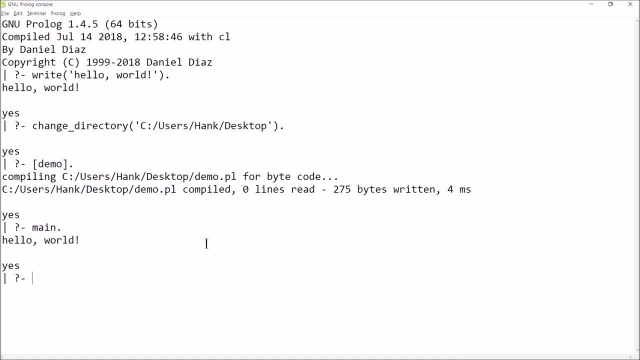 All right, So let's talk about some queries. Let's go back to the console, Okay, And let's reload. I'll just hit the up arrow Right, And I'll reload demo. Okay, And so everything got read just fine. 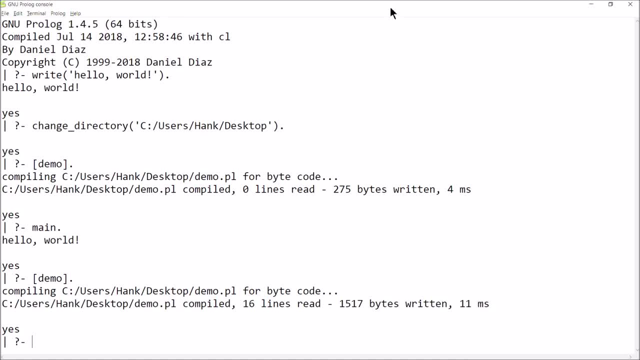 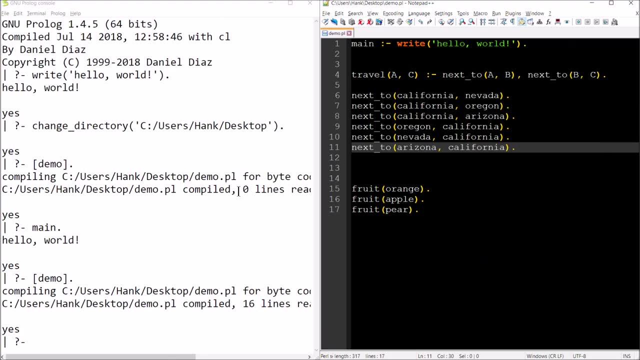 And so now what I can do, And I'll put this in one window to the left And then I'll put my Code Over here on the right, So we can just compare. Okay, So what I have is Is: I've got a bunch of facts in here. 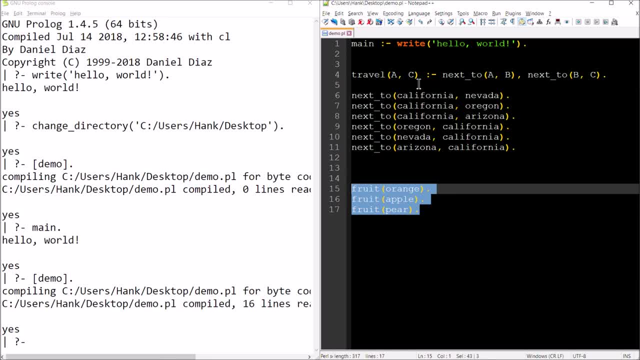 Line six through 11.. And then 15 through 17.. And then I've also got a rule on line four. Okay, So When I want to run a query, What I do is Is A couple of things. 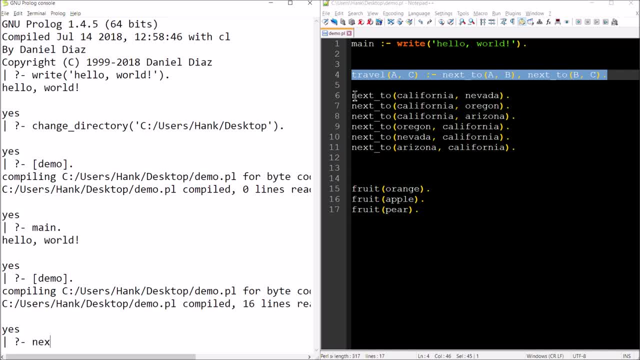 Okay, I can Query Right Typing in The name of one of the rules And I can say, All right, Well, It is California Next to Nevada, Right? So when I type that in And hit enter, 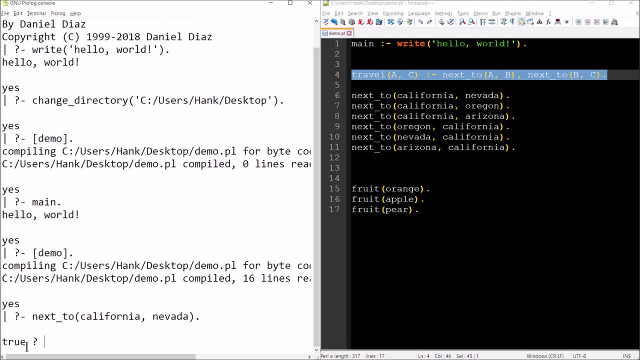 Right. I get a response Says true. So true Is Like Yes. What this says is: Yeah, Yeah, There are California's next to the Nevada. No problem Now When you're stuck here. and it says true. 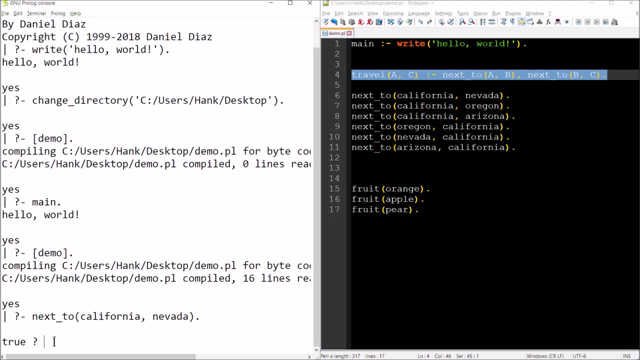 And there's a question mark. You know this says well, there may be additional answers. Okay, Now, what I wanted to ask was: Is it possible To get from California Nevada, Or are they Next to each other? 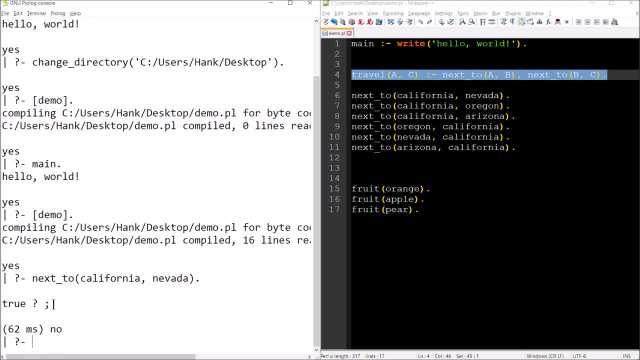 Fine Now if I hit Semicolon. Okay Now, The way that prologue is checking through all the facts. You know it was trying another approach, Through a depth first search, basically, And came up with no, And that's okay. 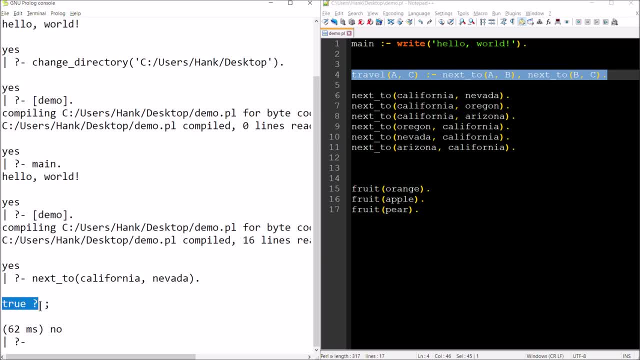 Right, Because I just wanted to know if it was possible, If it's true, that California is next to Nevada, And so I got the response that I wanted More on this- No thing here- In a subsequent video. Okay, So that's one way I can make a query. 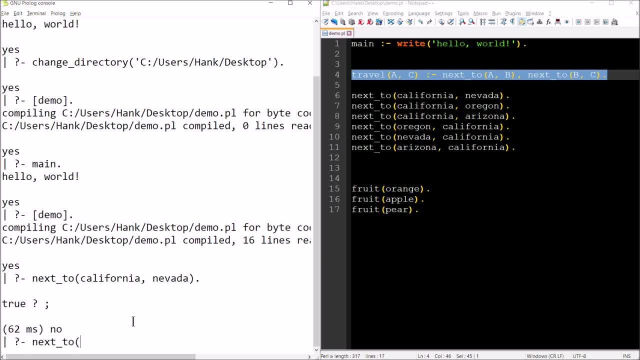 Another query that I could make would be to use a variable In The second Part of the line Right. So variables start with Uppercase characters. So I could say, all right, well, where are all the places that I could travel to? 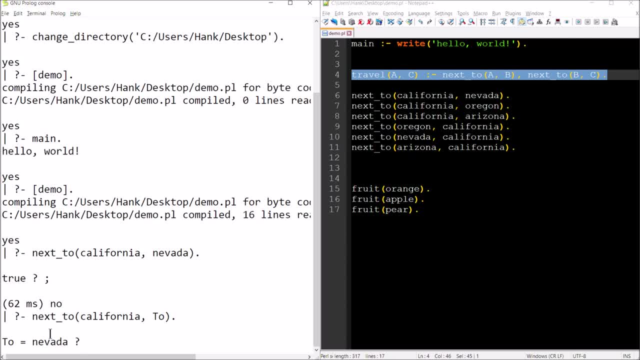 From California Who's adjacent? Okay, So you'll see now that the prologue inference engine goes through and says: oh well, let me take a look here. So you specify California And I have to go through and try to fill in the gaps for the two. 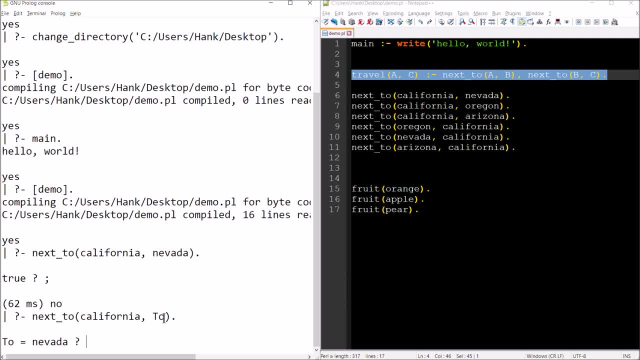 So California to Nevada, Oh yeah, Look, you can see right there on line six, Right? So I'll hit semi-colon And then that'll automatically advance me And prologue's now going to say: all right, well, also to Oregon. 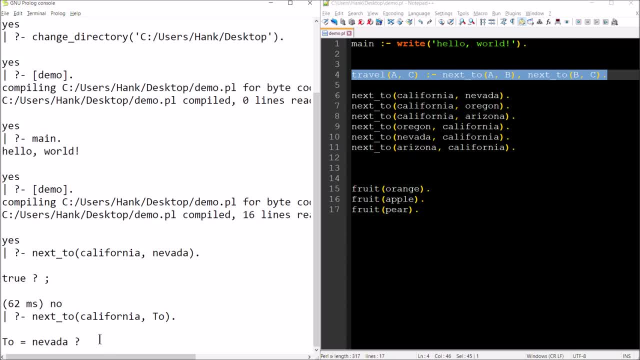 Right, So you can see line seven. There's a rule there, So I'll hit semi-colon to advance Right, And so then it'll say yeah to Arizona, And you can see That there's a rule there. 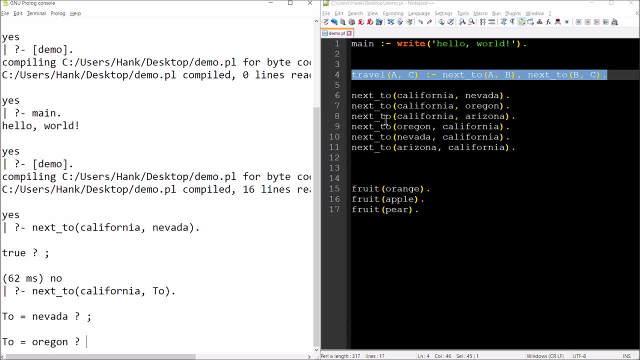 So I'll hit semi-colon to advance Right, And so then it'll say yeah to Arizona. And you can see That there's a rule there, So I'll hit semi-colon to advance Right, And so then it'll say yeah to Arizona. 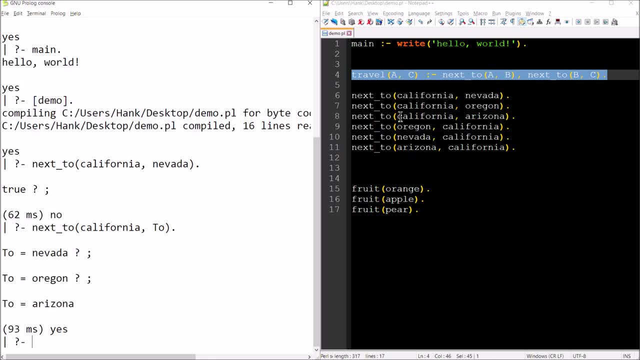 And you can see That there's a match Right. So California matches against line eight, And then there's Arizona, And then we're done Okay. So I can also Say: You know well, show me all the fruits that exist. 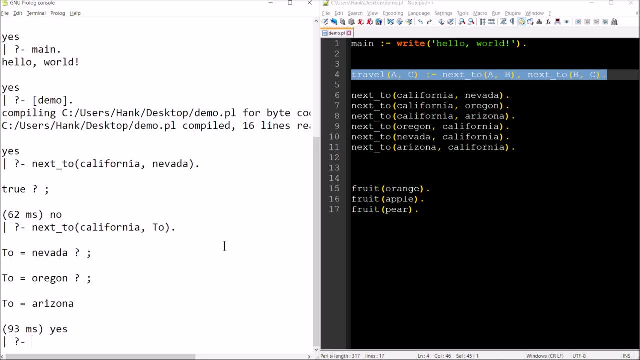 Right. It's because I put that in my knowledge base. So I could just say: well, show me All the fruits, And I could say, All right, So, All right, So, All right, So, All right. 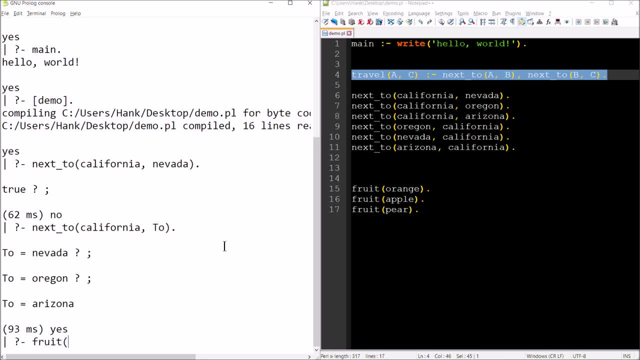 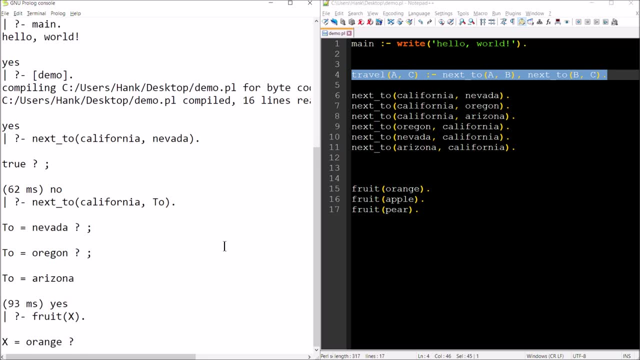 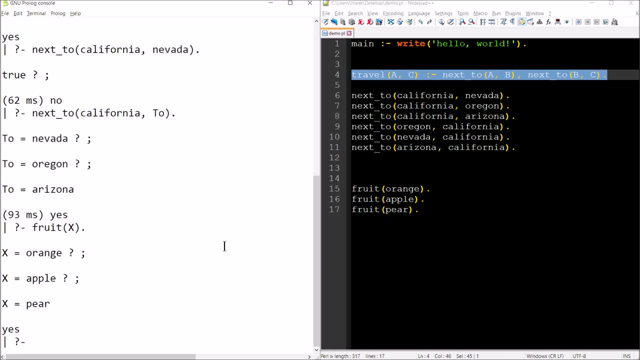 Right, And then I'll do period. Okay, So X is an orange. That's true. Right, That's one of the fruits. Apple, That's another one of my fruits in my knowledge base: Pear- Awesome, Okay. 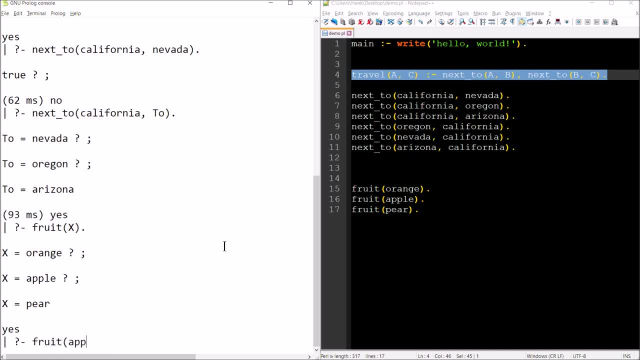 So I can also ask: Well, is an apple, According to my knowledge base, A fruit Right? And it's going to tell me: yeah, Right, here something that my knowledge base doesn't know about, so say like grapes, okay, well then, no right. so, yes, no, true, false. this is just letting me know, look. 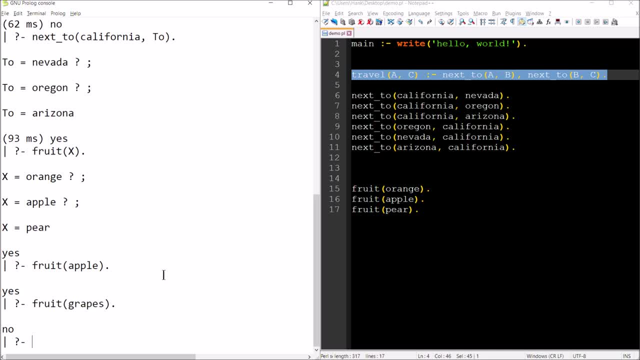 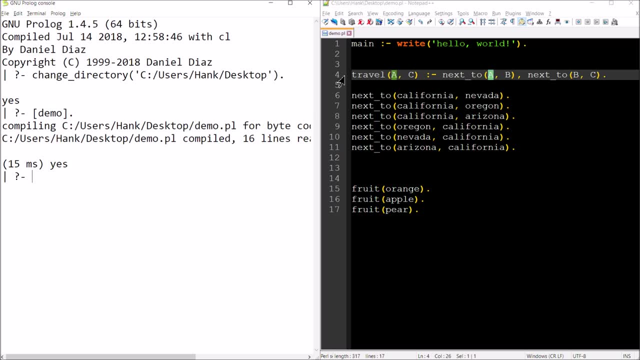 there's no entry. my knowledge base. I don't know what this is, right? so no, right, okay. so next up, I'm gonna try rule four, right? is it possible for us to go from, say, Oregon to Nevada? right, so what we'll do is is we'll put in here, we'll 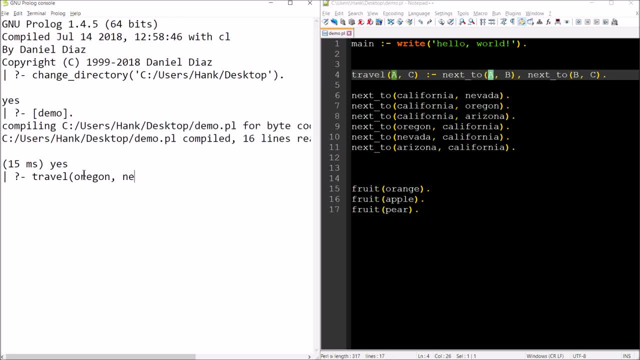 say, travel from Oregon to Nevada, okay, and so the result is true. why? because when I typed in travel, I'm trying to engage the rule on line four right, and so when I do that, Oregon basically becomes. if you take a look at this, I'm trying to engage the rule on line four right, and so when I do that, Oregon basically becomes. if you take a look. 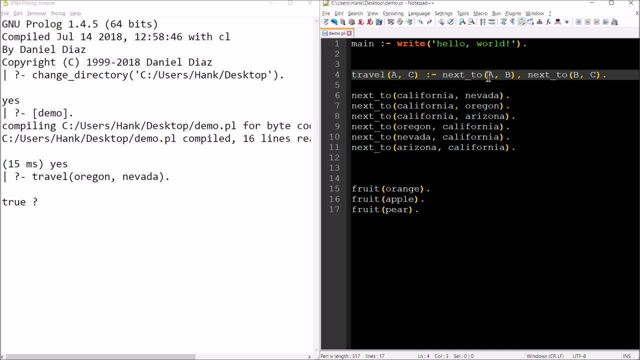 on the right hand side here, the if part becomes, takes the place of a, and then prologue goes through and says: all right, well, from Oregon where can I go? well, I can go from working to California. so California becomes B. and then the second next to starts off with Oregon as- or, excuse me, as California's B. and so then, 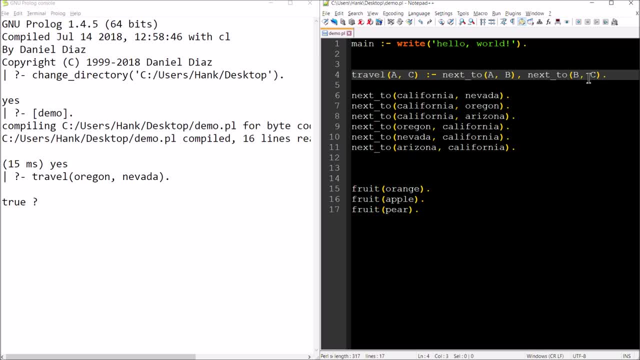 on the, the second part of the expression, the next two from, for B and C. it basically that says okay, well, from California is there a match for Nevada, and so there's a match for Nevada. there is, because of fact, six okay, and so true response was possible, true and 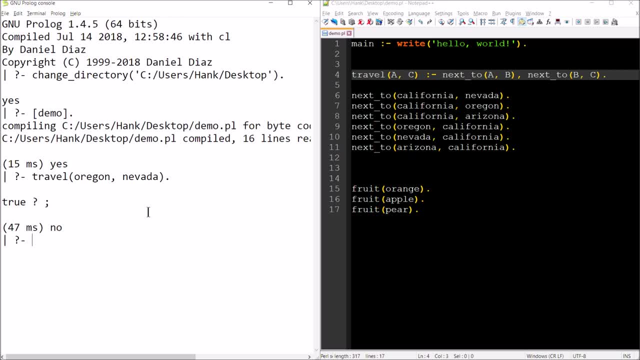 says: okay, yeah, no problem, you can, you can travel there, you know? and then we're finished, we've, we've, we've verified that we can actually move from Oregon to Nevada. now what would it look like if I can't? well, let's see, here can I travel. 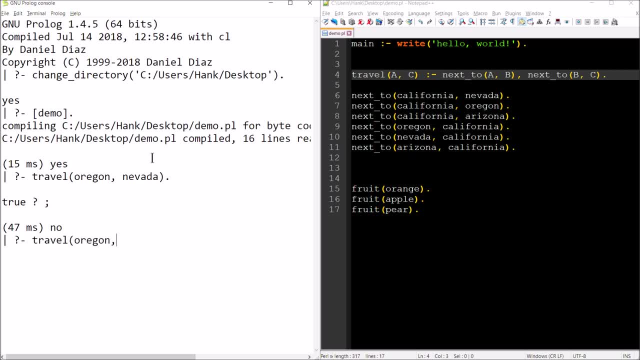 from you know Oregon to Maine, right? so what's that gonna say? no, there is. no, there is no main in my knowledge base, right? and so this rule can't find a path. there is no fact main that says that you know from may even exists in my world, in my, in my knowledge base here. okay, so last thing, 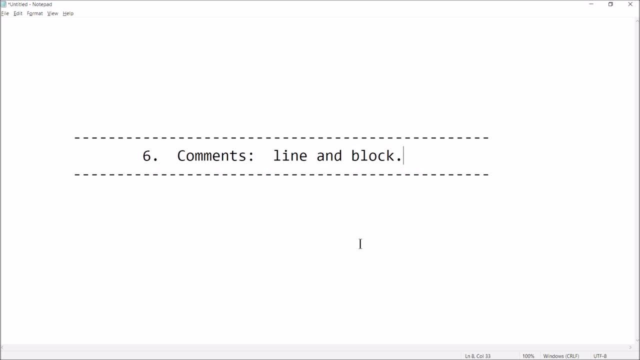 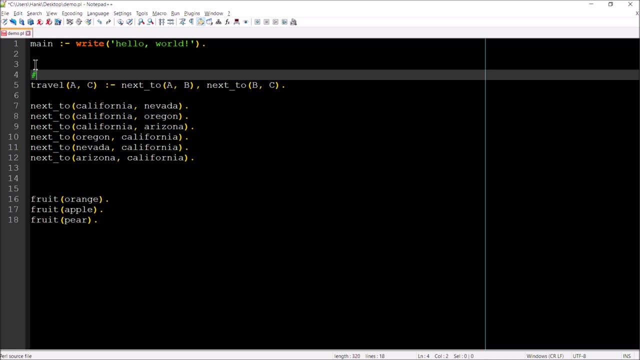 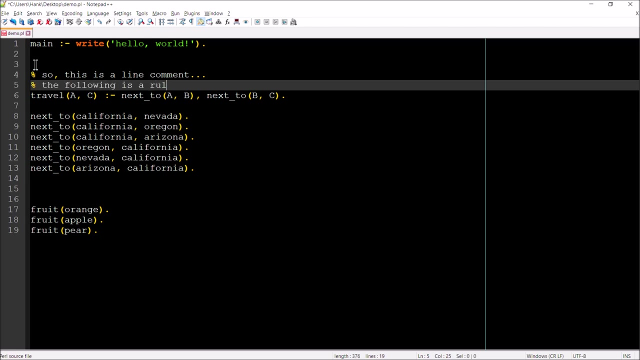 I want to do in this video is just show you the basics of comments, right. so line and block comments: line comments in prologue with a percent, right. so this is a line comment and so if I wanted to specify that, okay, this is the following: is a rule, right? can I get from point A to? 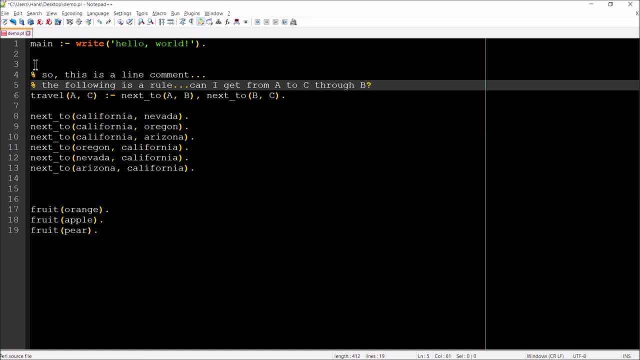 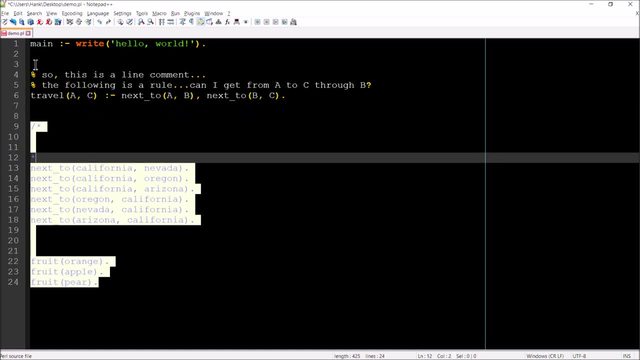 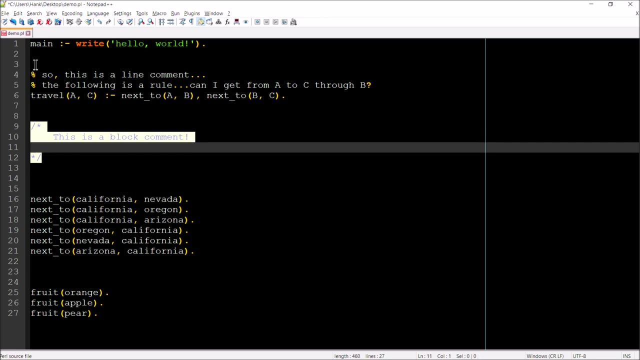 point C through B. this is basically what this rule allows me to do right now. if I want to do, block comments, and they're you know what you, what you're used to, right. so forward slash, star and star, forward slash. this is okay. so the following lines: these are your two options. okay, so let's go ahead and 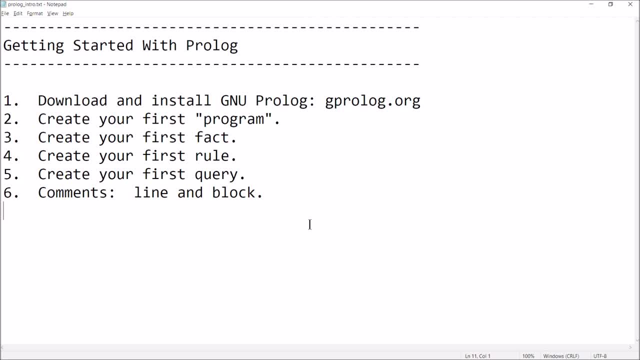 summarize what we talked about in this video. in this video I was hoping to just get you started right. I wanted to show you how to go and download, you know, a copy of prologue. get that thing installed. I wanted to show you how to create your very first.